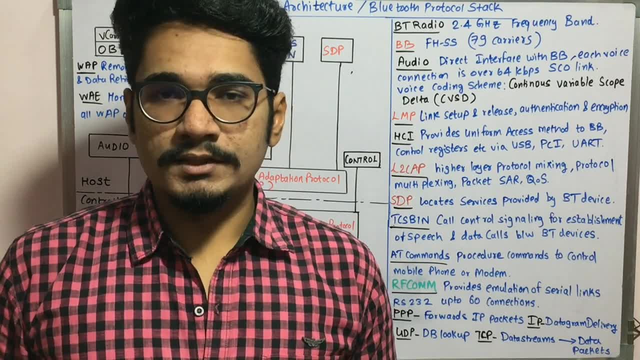 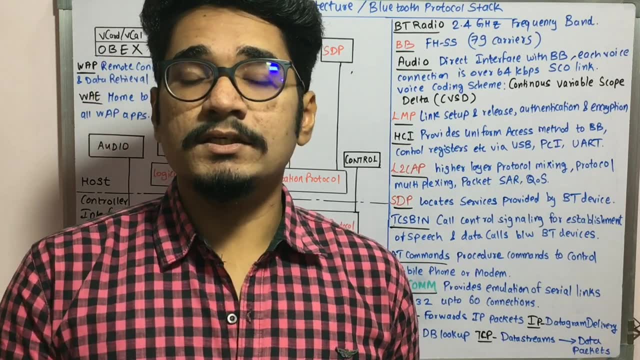 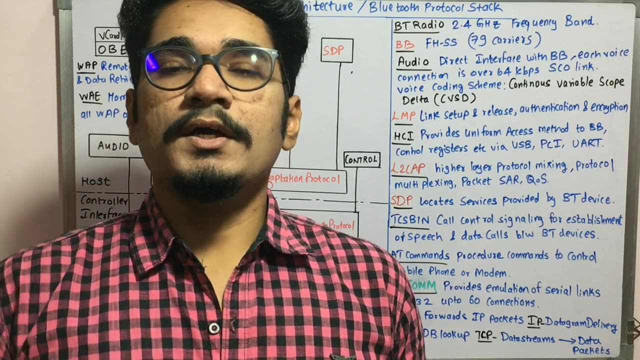 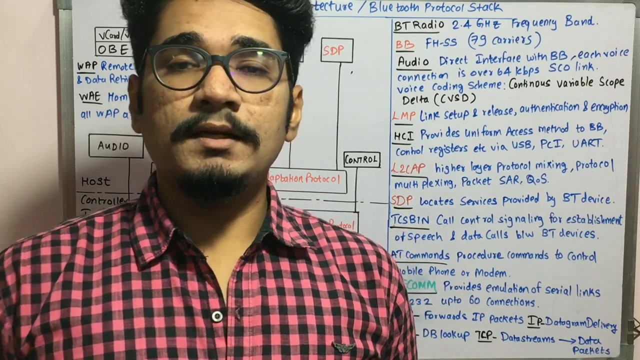 HSS technique, which is mainly done for efficient bandwidth utilization, And also in this you have two major physical links- that is called as a synchronous connection oriented- as well as the asynchronous connection- less links. And so when packets are sent in SEO- that is, synchronous connection oriented- it is used for audio only transmission or you can use combination of both data as well as audio, Whereas if you use ACL packets or when ACL links are used, packets are sent only for data only transmission. 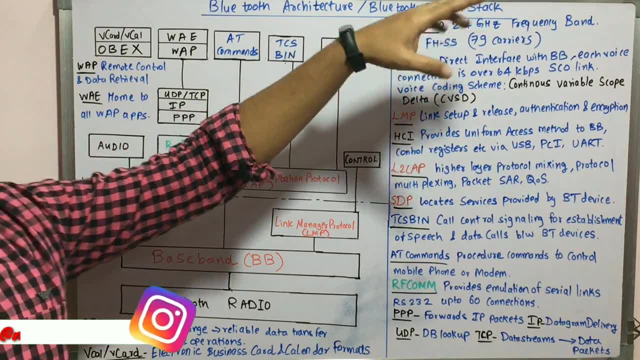 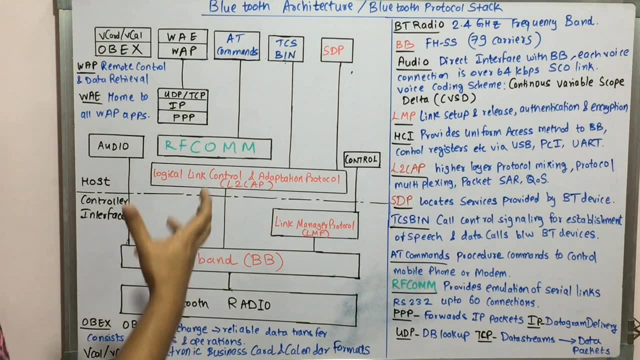 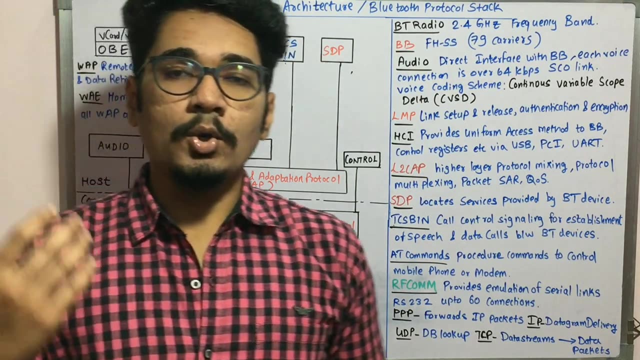 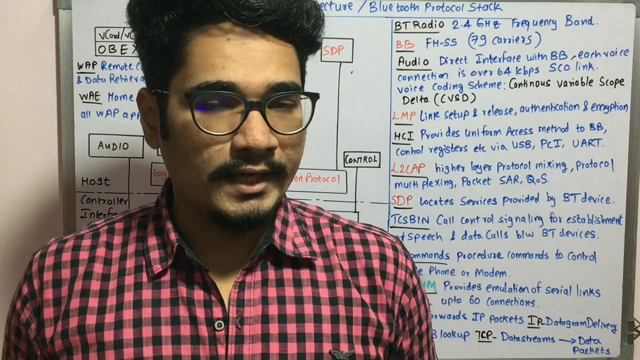 So next, in Bluetooth radio it specifies: or the Bluetooth operates mainly within the 2.4 gigahertz frequency band, Then a layer above you have the baseband. So written in red are the Bluetooth core protocols. So baseband majorly specifies: or it handles all the lower level operations, that is, at the bit level or at the packet level, And so some of the operations include forward error correction, FEC, and cyclic redundancy checks, CRC. Then you have automatic repeat request, ARQ. 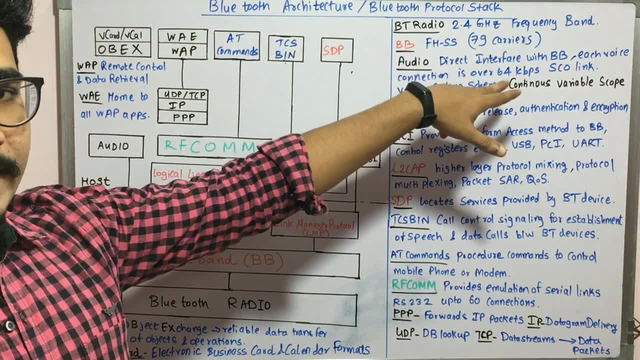 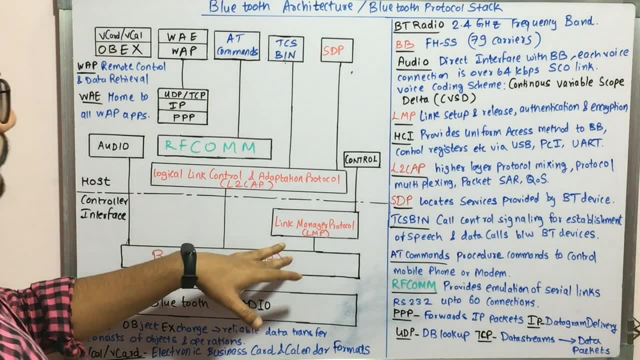 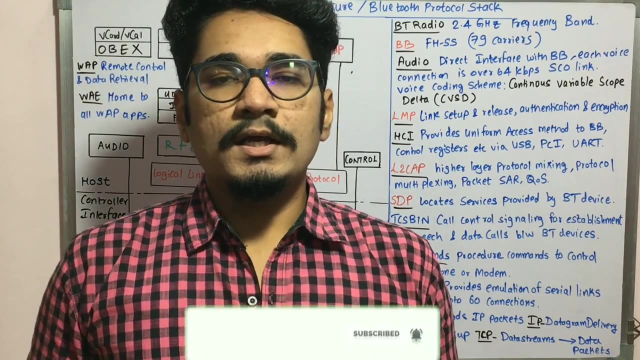 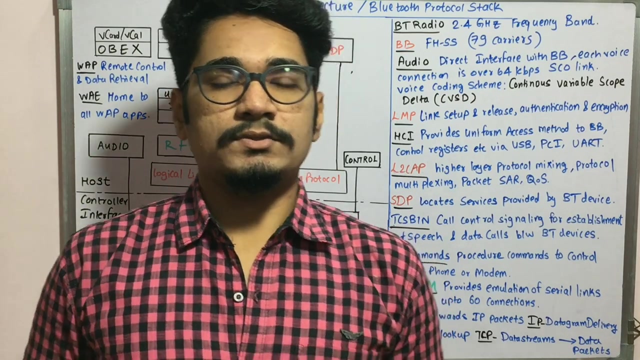 As well as encryption, And so it has got 79 carriers and it uses the FHS, that is, frequency hopping, spread spectrum technique. Next we move on top of this, that is, we have the link manager protocol. So link manager protocol establishes the configuration link among various devices. For example, consider: a fitness tracker is there which is Bluetooth enabled, And then you have a Bluetooth speaker and then you have a Bluetooth handset. So the devices when they form a Pico net together. So basically the 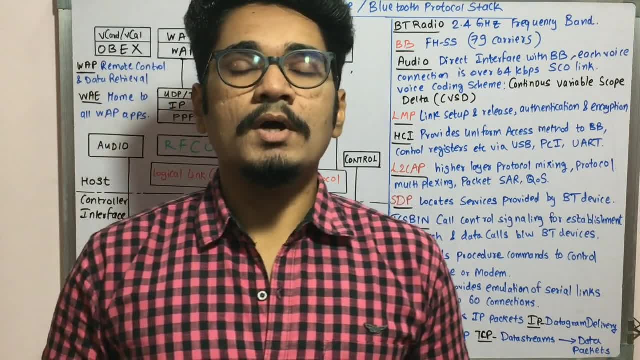 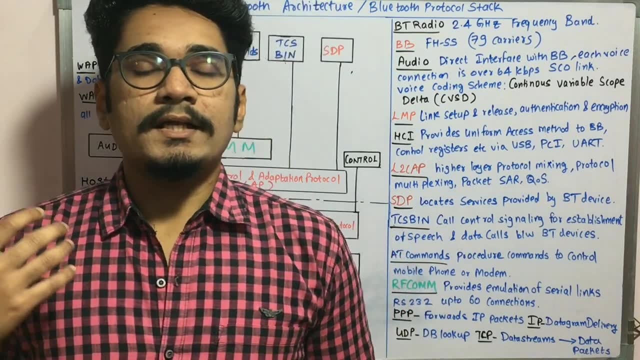 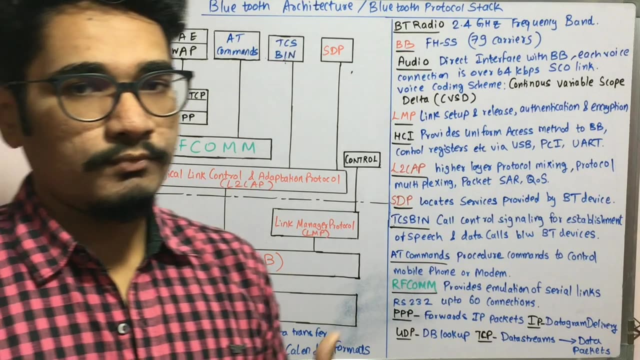 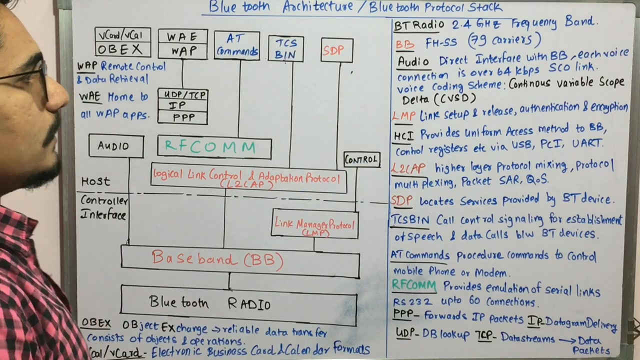 connection establishment is done with the help of LMP, and also, after their use or after their intended purpose, the connection is released. It also manages the traffic scheduling and it also does the authentication as well, And then it does the power management. So all those functions are mainly taken care with the help of LMP, And so it has got a controller that is the LMP controller. So that is this additional block which you can see here. Next you have this audio. So audio is a hardware which 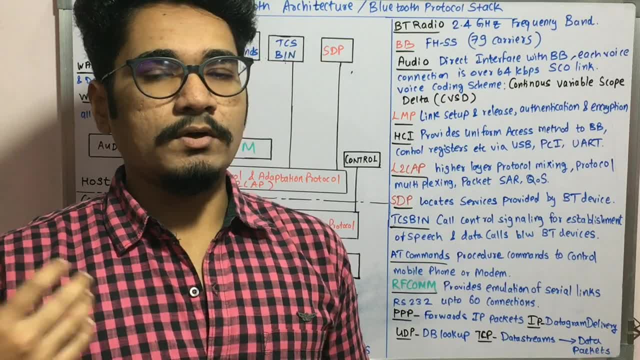 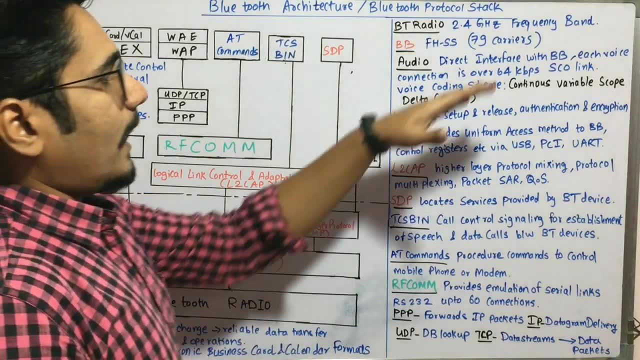 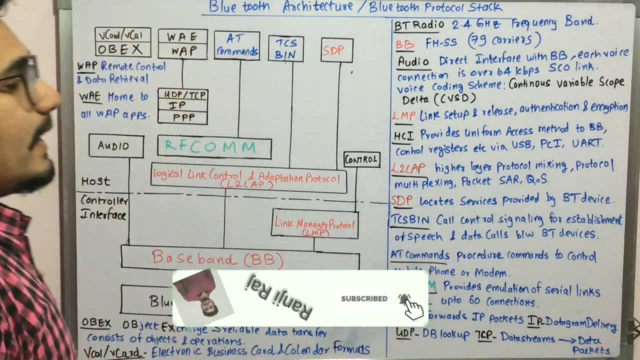 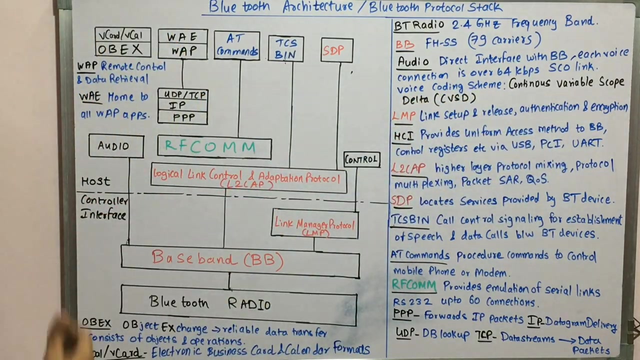 is put in the Bluetooth in order to just receive the files or in order to just play some music or songs. So it is directly interfaced with the baseband, that is BB, and each voice connection is over the 64 kbps SEO, that is, synchronous connection oriented link, And the voice coding scheme mainly used in this is continuous variable scope delta. that is called as the CVSD. Next, we have an interface that is called as a host controller interface, So it sits between the 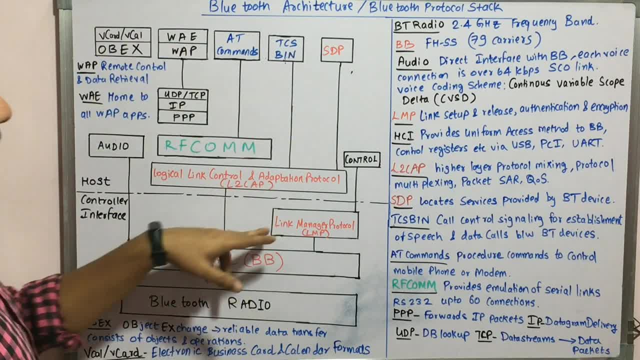 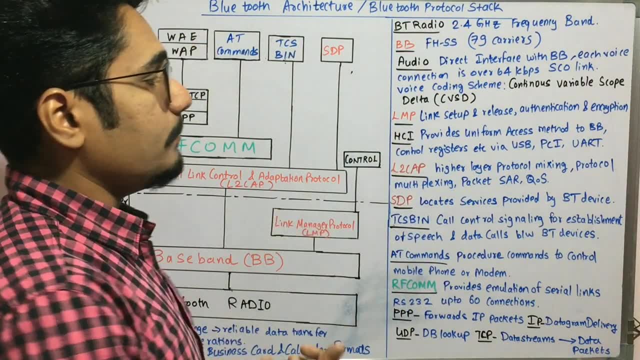 logical link control, that is LECEmple, And then you have the at the connection manager, that is at the link manager protocol, LMP. So HCI mainly provides a uniform access to the BB. that is basement, and it controls various registers, that is hardware registers, and it is done via. 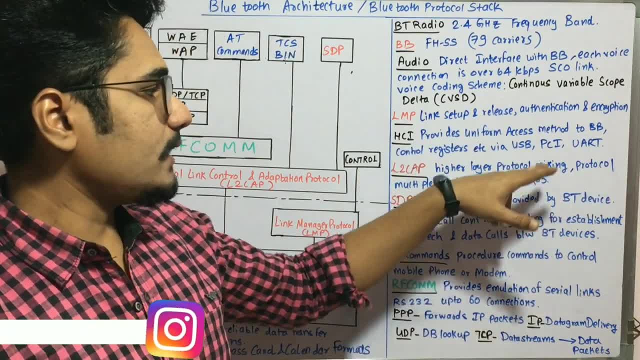 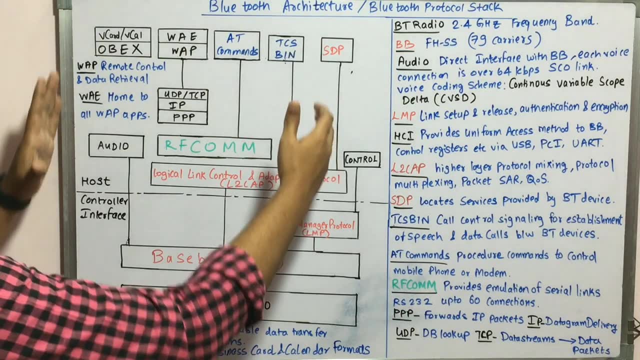 That is USB. then you have PCI, that is peripheral component interconnect, and then you have a UART, that is universal asynchronous receiver as well as transmitter. Next you have this one big code protocol, that is we, which is called as the logical link, control and adaptation protocol. 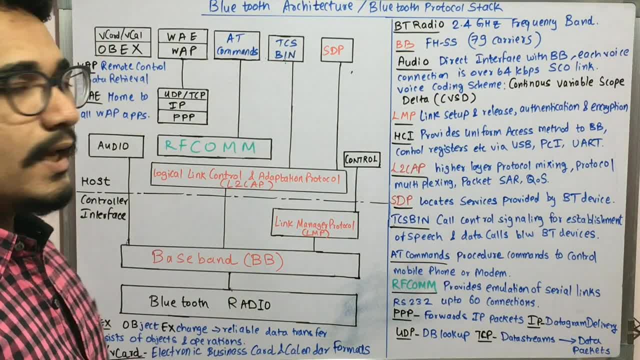 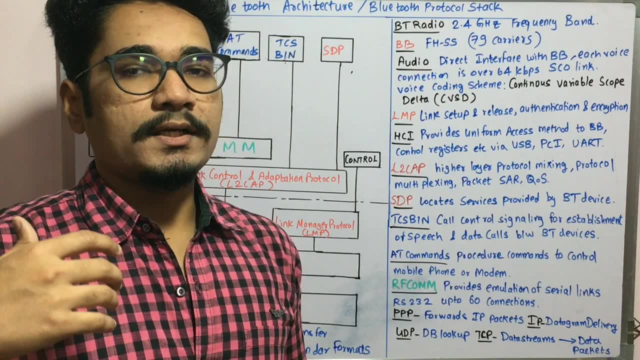 So this we also saw in the WPAN protocol. So this again forms a Bluetooth core protocol in this. so it majorly deals with the higher layer protocol mixing. it manages or it adjusts all the upper layer protocols. that is this portion and it mainly deals with. 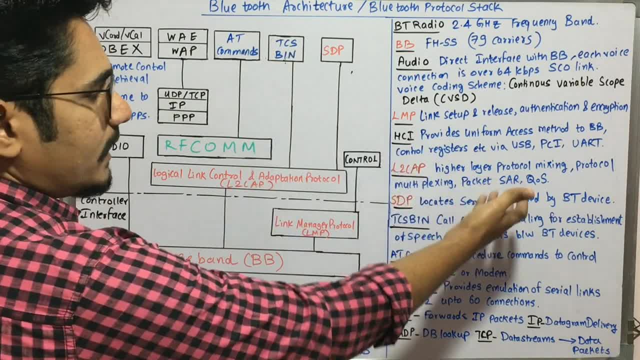 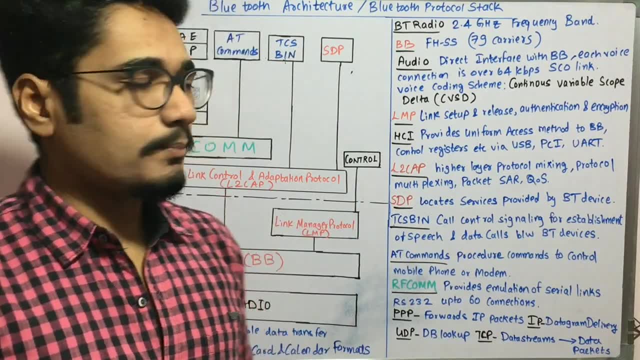 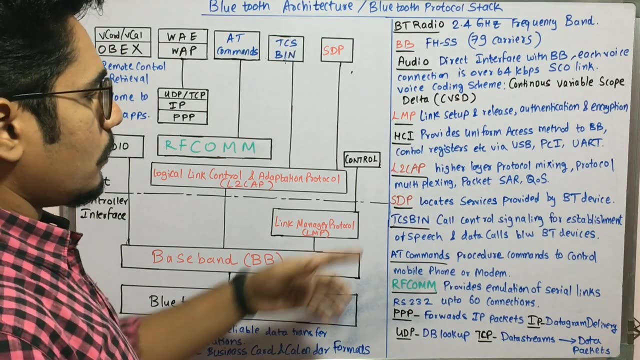 protocol. multiplexing, then packet segmentation and reassembly, called as the SAR, means large packets are divided into small, small pieces of smaller bytes and then it is done for further processing and then you have the quality of service. Next we move on to the last core protocol, that is, we have the service discovery protocol, that is 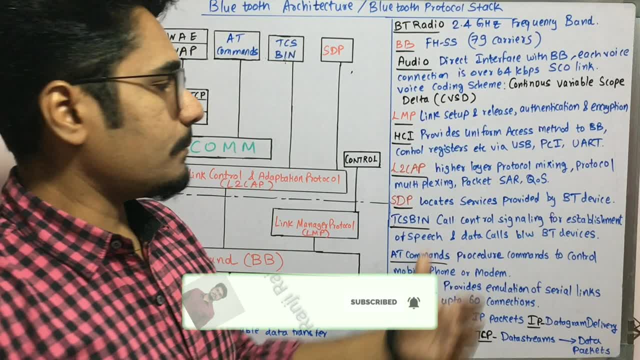 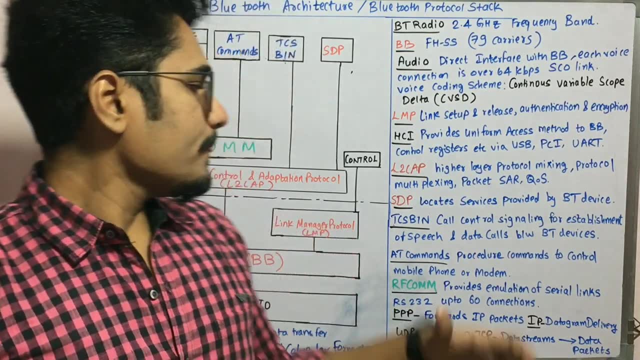 called as the SDP, and it locates different services which are provided by that particular Bluetooth device, Its MAC address, its device address, its number of pairing devices, etc. So all those are managed with the help of SDP. Next we move on to some 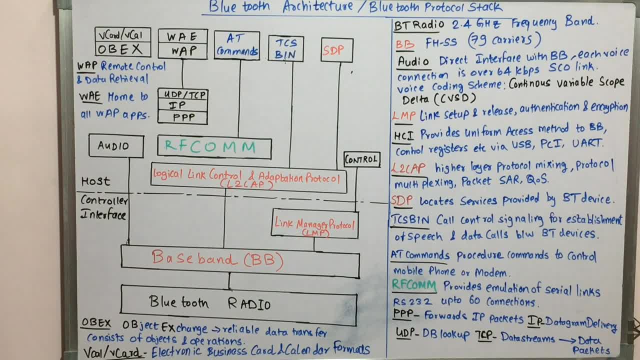 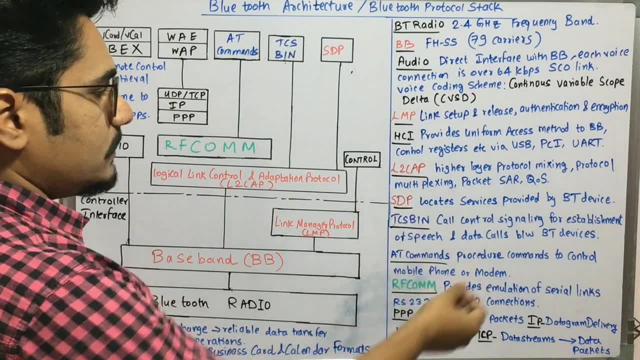 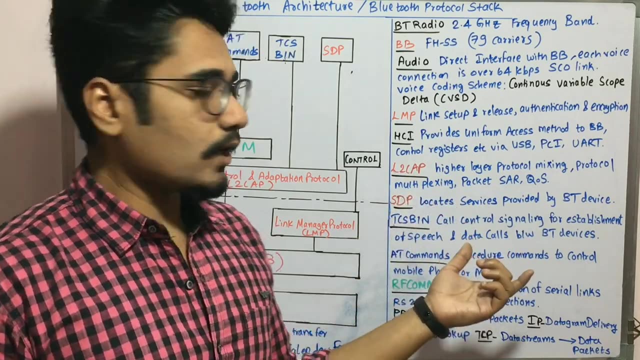 telephony control protocols. So we have two telephony control protocols, that is, we have the TCS BIN, so that is called as the telephony control specification binary. so that is written as TCS BIN and it controls call controlling and it is used for establishment of speech as well as the data calls. 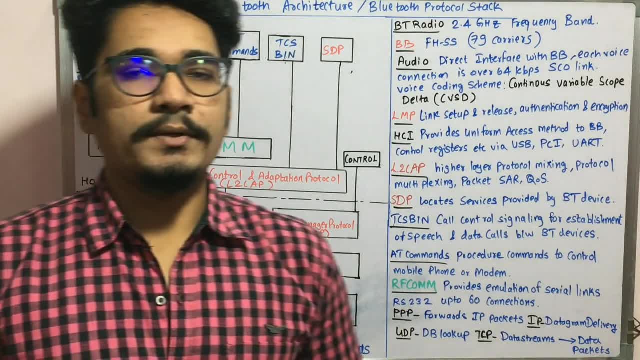 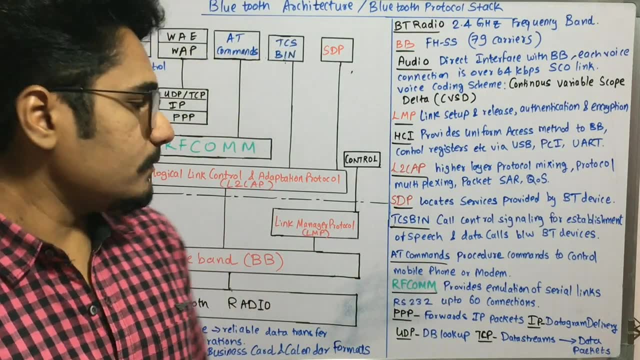 and it is done with the help of various Bluetooth devices. So whenever you connect different Bluetooth devices to your car system or audio system, you have hands free mode. so that is mainly done with the help of TCS BIN. Next we have the attention commands, or the attention sequence. 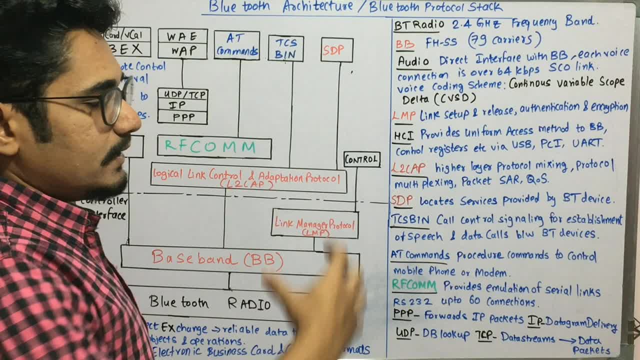 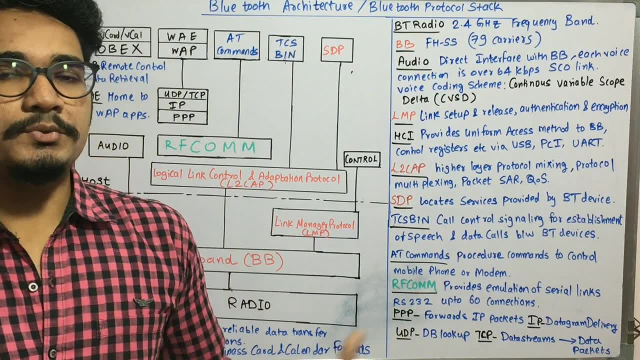 commands called as the AT commands. So it basically has a list of commands or a procedure to control a mobile phone or a modem. So various kinds of shell level commands are there which is used to control your mobile phone, which is there remotely or some other stereo. 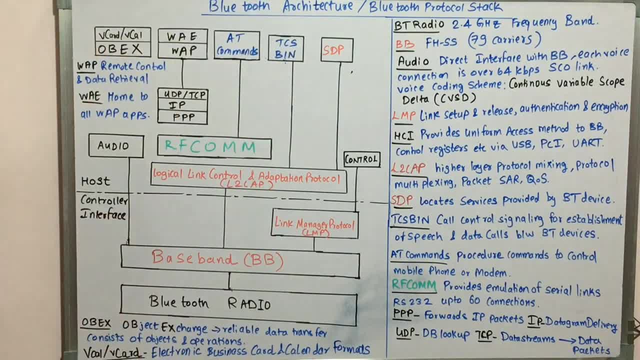 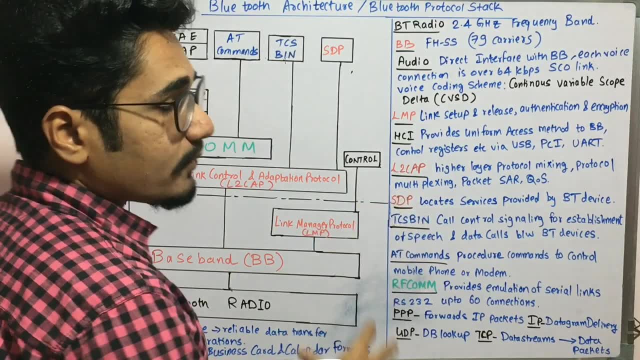 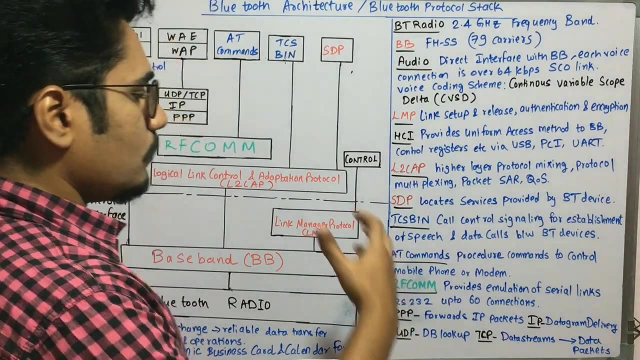 system or some cockpit kind of things. Next you have this cable replacement protocol, that is, you have the radio frequency communication. it is called as the RFCOM, So it mainly provides the emulation of serial links, that is of recommended standard 232 and it is up to 60 connections. So 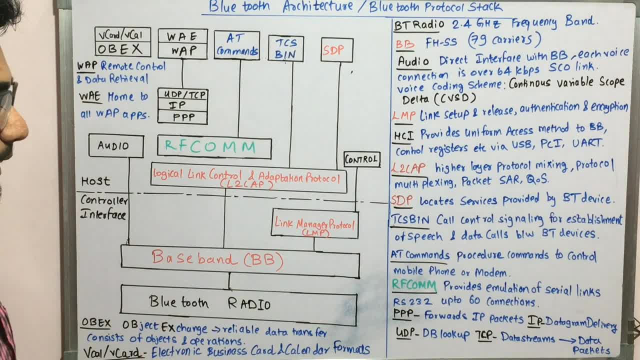 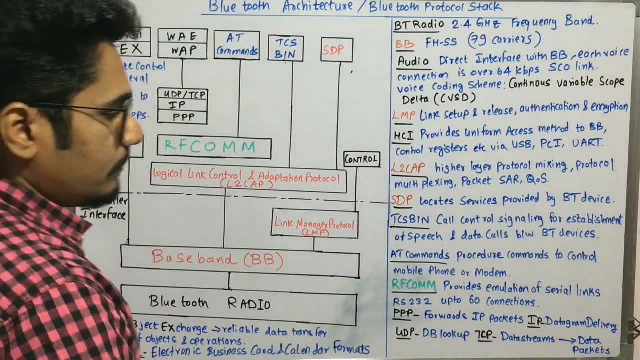 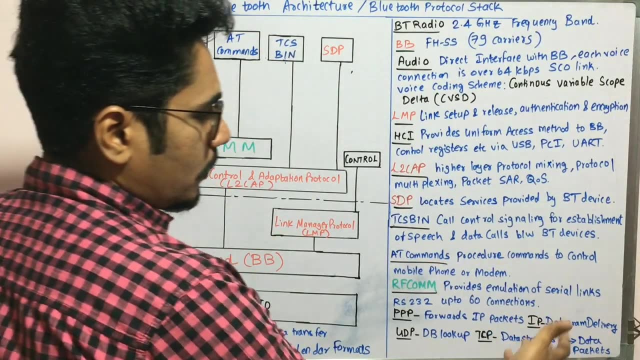 this is the only cable replacement protocol in the entire Bluetooth architecture. and next you have some adopted protocols. So those are. you have the point to point protocol, that is triple P, So it forwards mainly the IP packets to the LAN network. Then you have the IP, that is the internet protocol for. datagram delivery on the routers. Then you have the user datagram protocol. It is mainly used for a database lookup. Then you have the TCP, that is transmission control protocols. It mainly deals with converting the data streams to data packets. Then you move little. 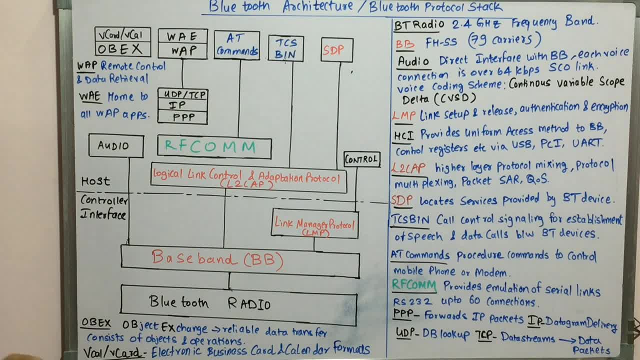 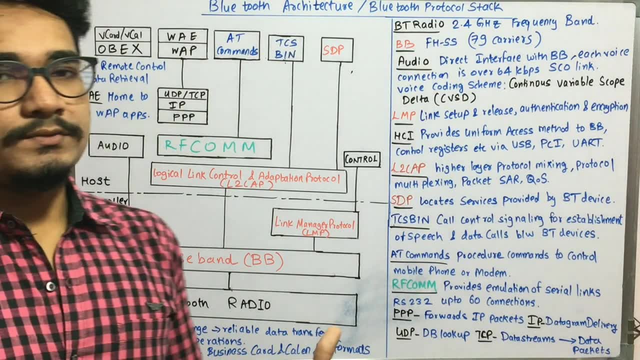 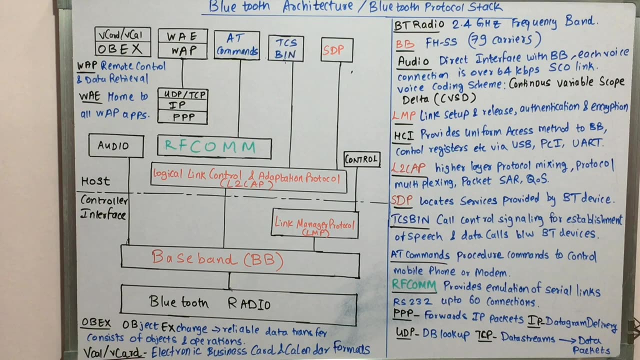 upper. that is, you have the WAP, that is wireless access protocol, that is, it mainly deals with the remote control and data retrieval of various devices when you do the transfer between PC to a mobile phone and you have this WAE, that is wireless application environment, where 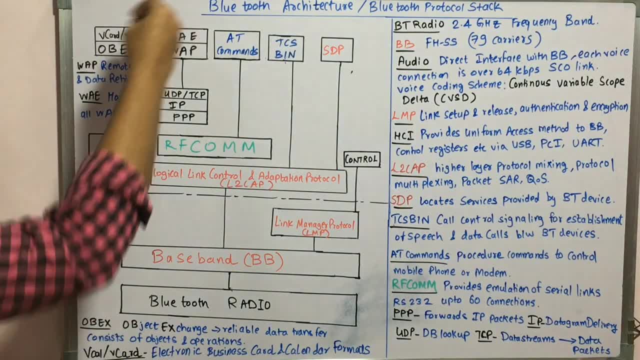 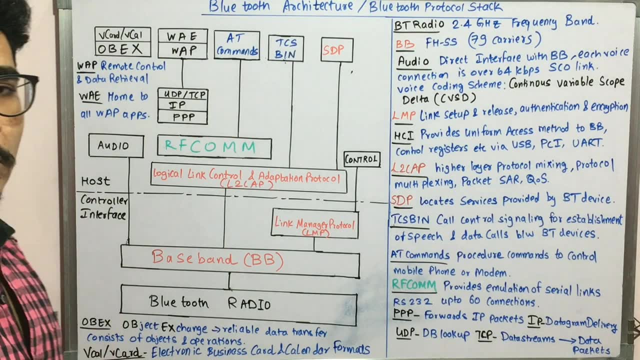 it provides home to all WAP applications which are hosted in this. Then when you move little this side, you have this OPEX. so OPEX is a major technology which is used in most of the Bluetooth, that is, from Bluetooth 2.0 to the latest. 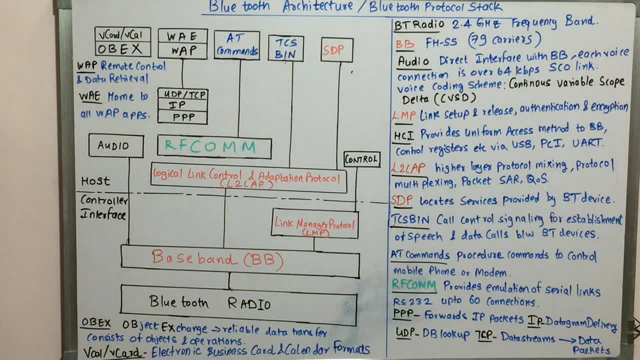 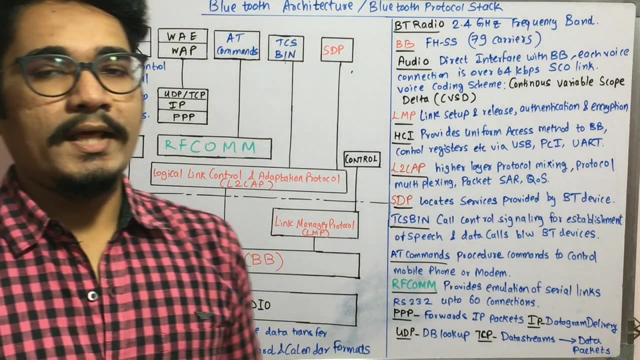 version of Bluetooth 5.0. So it stands for object exchange. So from the name itself, it is mainly used for exchanging different kinds of objects. So it provides reliable data transfer between various systems and it consists of certain things called as objects as well as operations, So this can be understood like in: